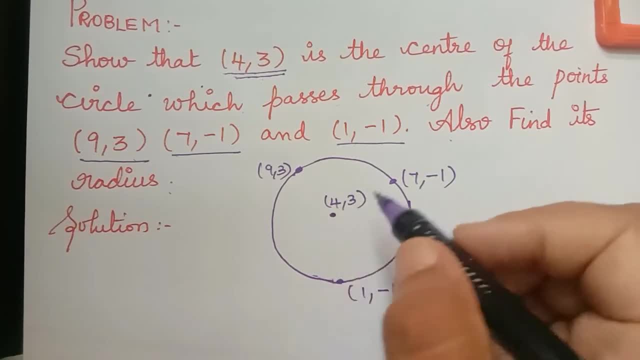 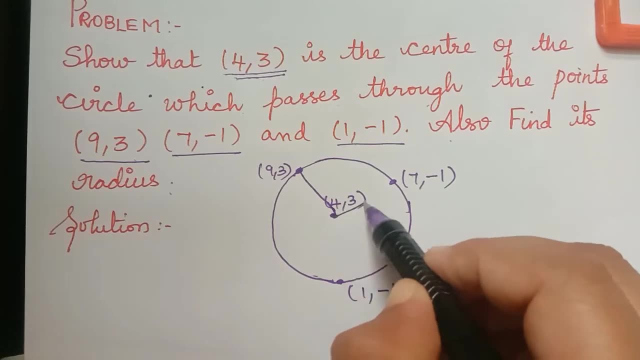 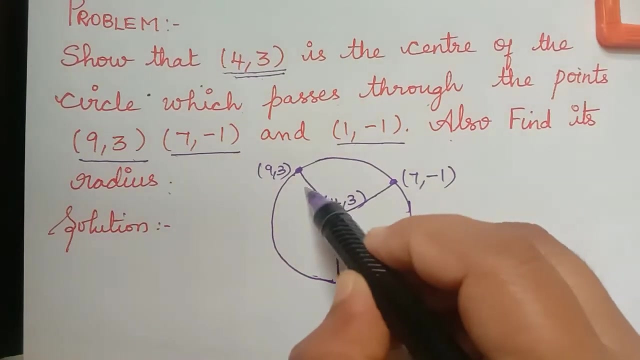 So to prove that this is the center, we have to prove that the distance between this point and this point will be equal to the distance between these two points and that distance will also be equal to the distance between these two points. So if we prove that these three distances are, 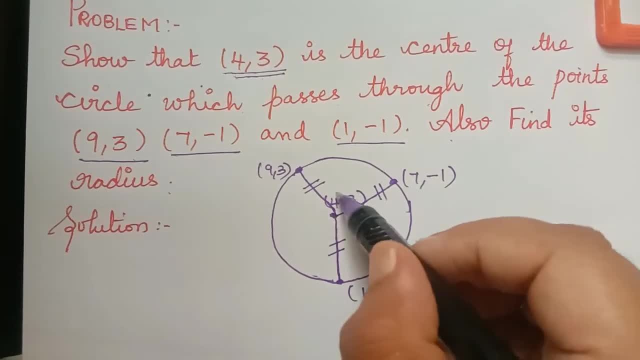 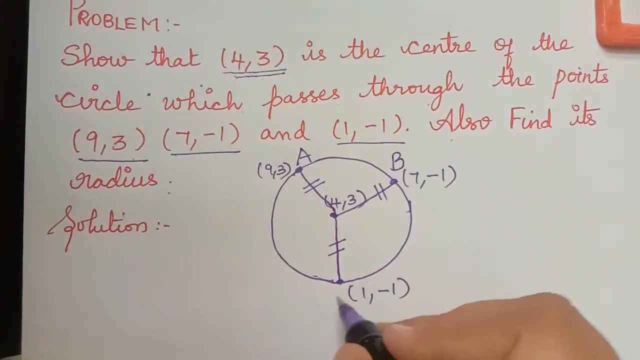 equal, then we would have proved that 4 comma 3 is the center of the circle, and hence we can also obtain the radius of the circle by this. So first we will name the points. So let us take this as point A, So let this be point B and this is point C, and let us consider the center to be: 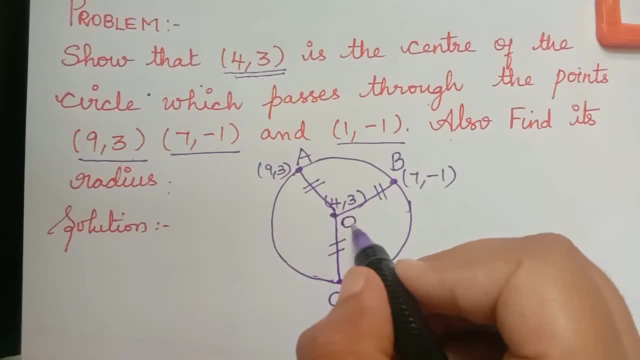 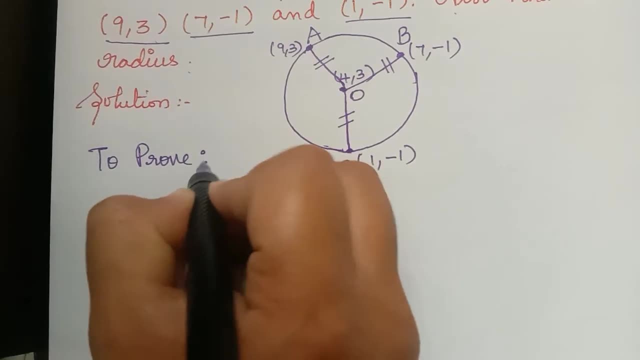 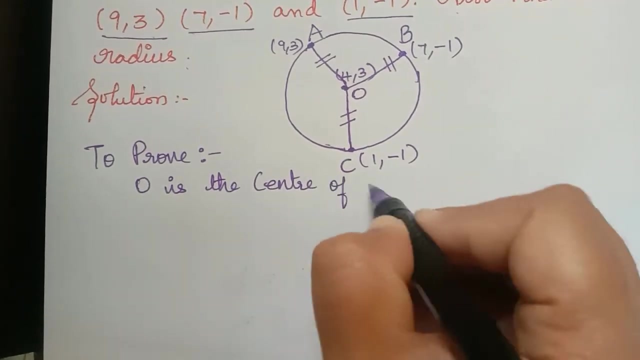 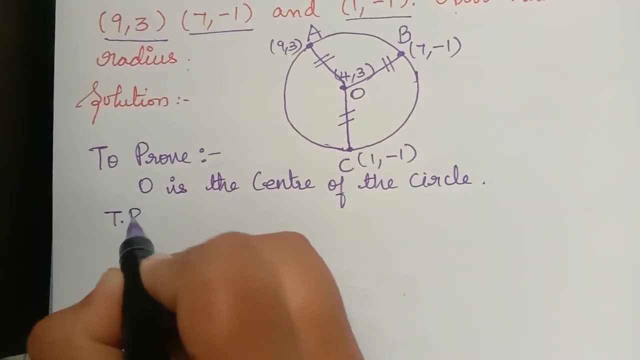 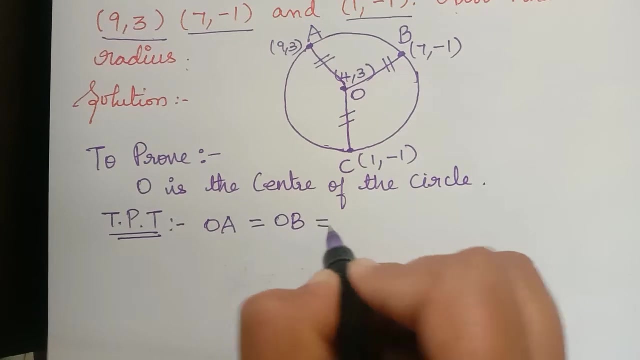 O. So first let us prove that 4 comma 3 is the center, for which we have to prove. So we have to prove that O is the center of the circle. So in order to prove that O is the center of the circle, for which we have to prove that, So to prove that OA is equal to OB, is equal to OC, We have to prove. 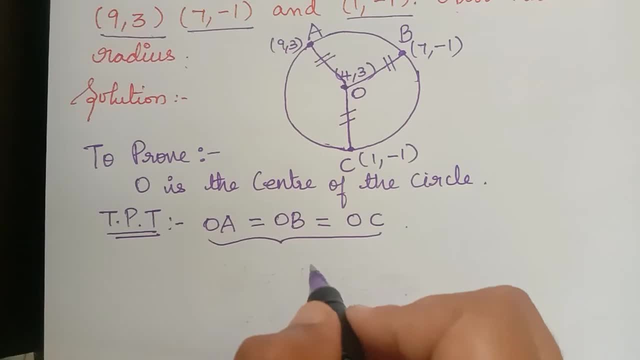 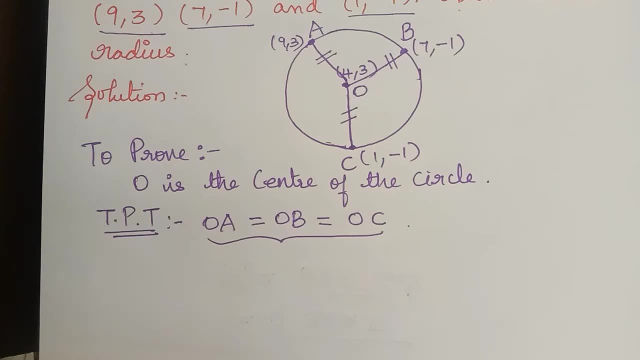 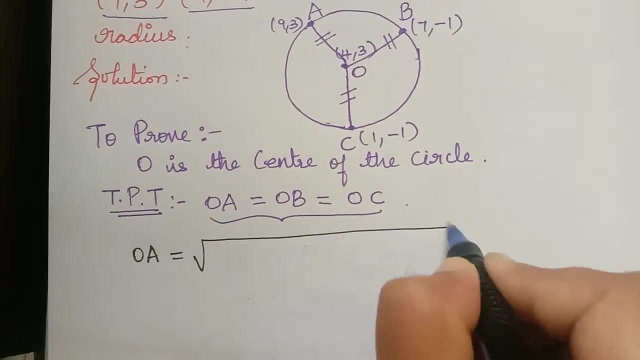 that these three distances are equal to one another. So let us first find out the distance OA. So how can we do that? We have to find that by using the distance formula. So now here, OA will be equal to square root of. So now here we are using the distance formula, So this will be in. 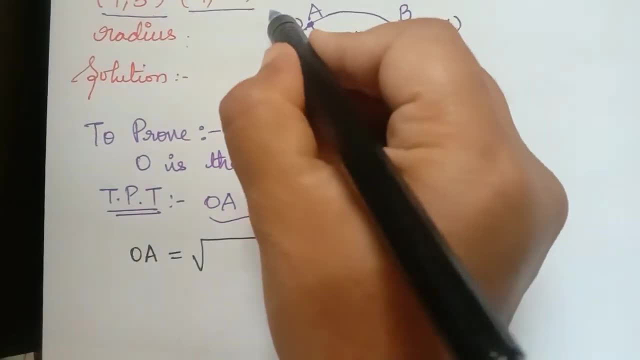 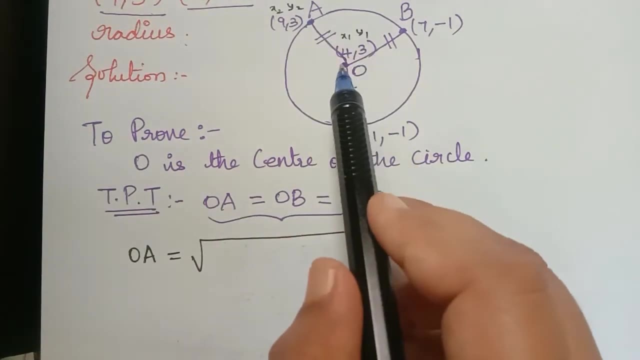 that case X1- Y1 and this will be X2- Y2.. So by the distance formula we know that the distance between two points is equal to square root of X1 minus X2- Y2.. So this is the distance between two points. 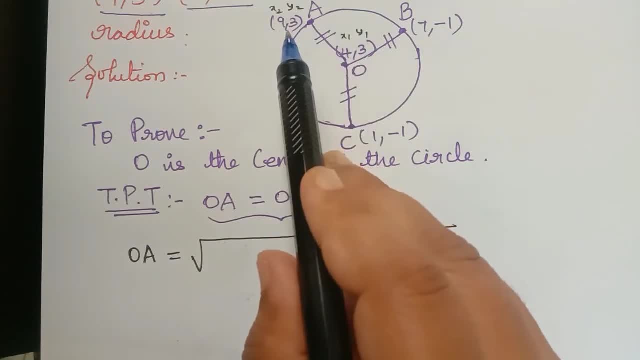 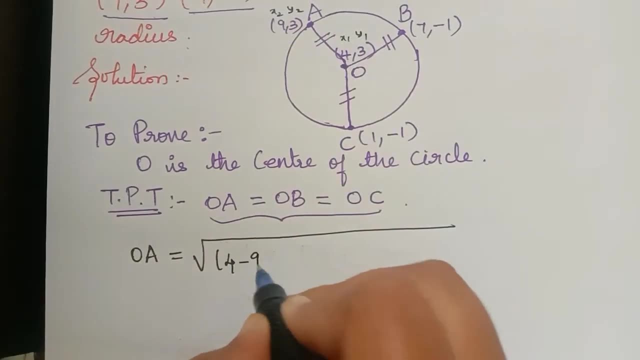 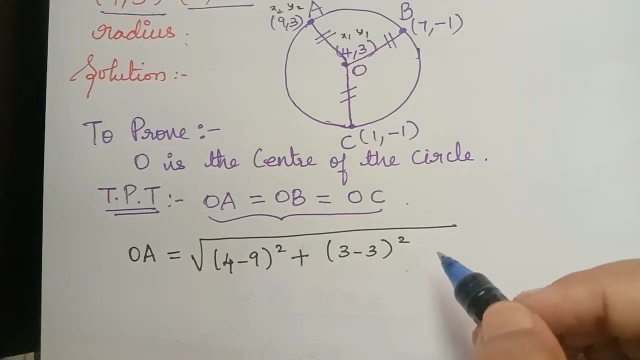 So this is the distance between two points. So we have to prove that this is equal to square root of X1, X2, Y2 plus Y1 minus Y2, the whole squared. This is by the distance formula. So, using the distance formula, we obtain 4 minus 9, the whole square, plus 3 minus 3, the whole square. So simplifying this. 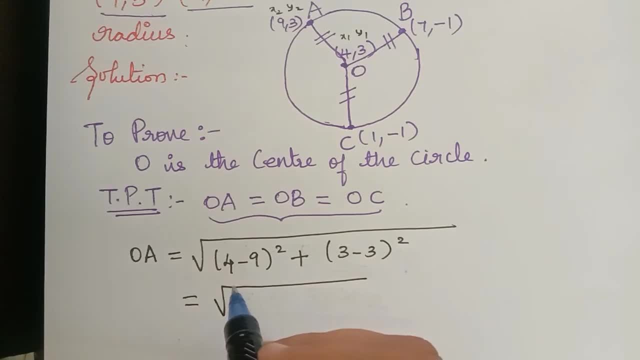 this will be equal to square root of what is 4 minus 9?? It is 5.. So minus 5 actually. So minus 5 the whole squared, plus 3 minus 3, the whole square. So this is by the distance formula, So. 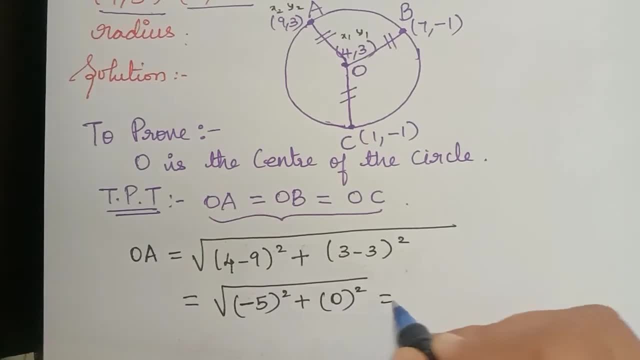 minus 3 is 0, so 0 squared so that will be equal to square root of minus 5. the whole, squared minus into minus, will become plus 5 multiplied with 5. so square of 5 is 25 and plus 0 is 0, like it will. 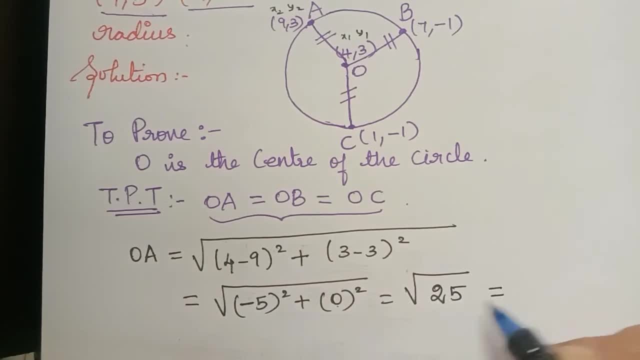 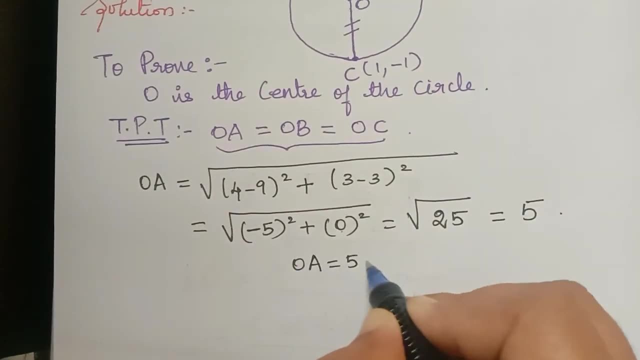 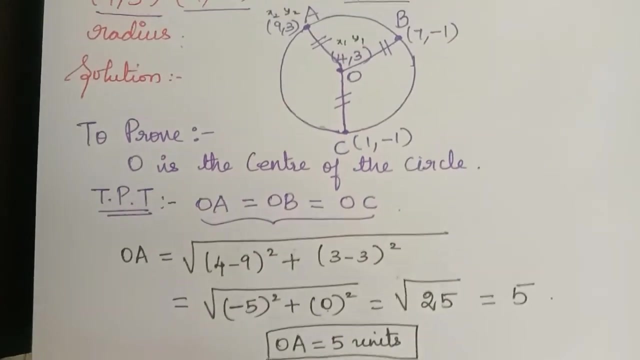 be only 25 here. so what is square root of 25? it is equal to 5. so we have obtained o a to be equal to 5 units, so let us just mark this. after this we have to find the distance ob now here: x1, y1 will. 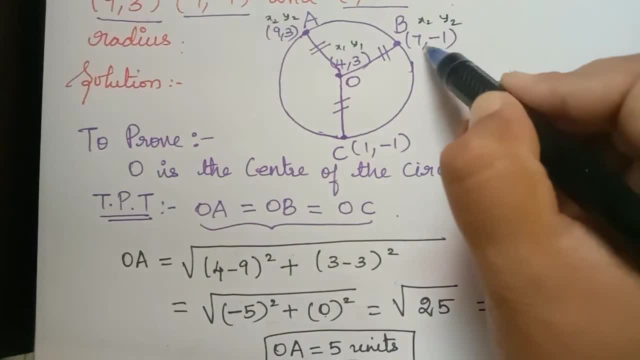 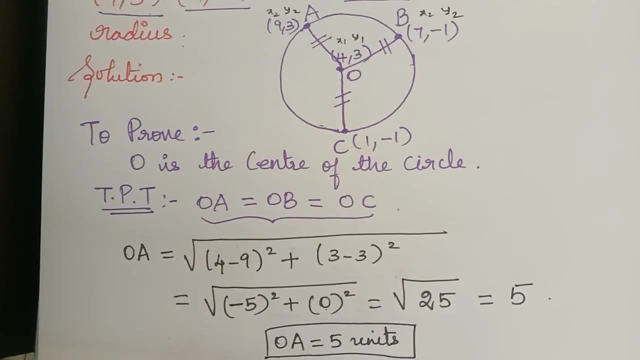 be 4 comma 3. in this case x2 and y2 will be 7 comma minus 1. so now let us find ob. so ob will be equal to square root of now. what is that? 4 minus 7, the whole squared plus 3 minus of. 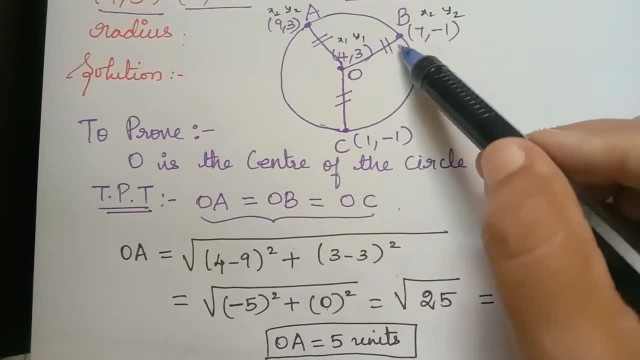 1, so that will be equal to 4 minus 7 the whole squared, plus 3 minus of 1, so that will be equal minus 1 the whole squared. so let us do that. so ob is equal to square root of first is 4 minus 7. 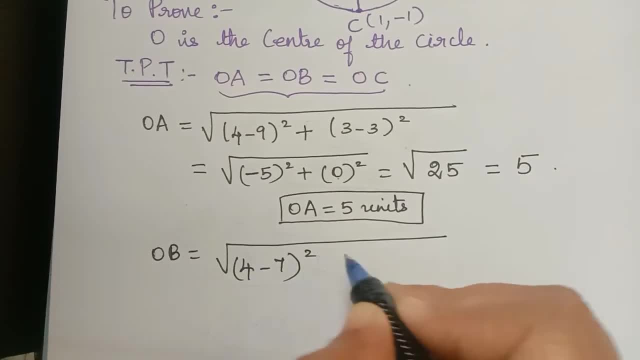 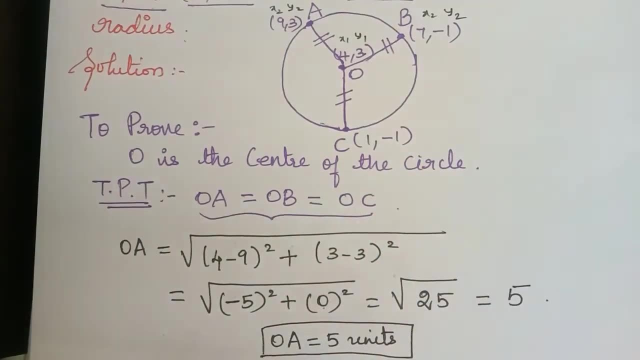 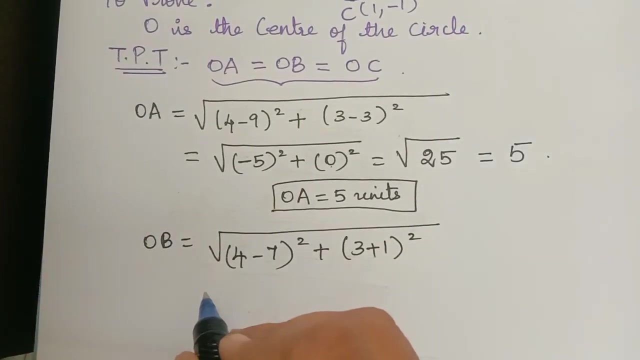 the whole squared. so 4 minus 7, the whole squared plus. so what is the y coordinate here? 3, so 3 minus of minus 1. so that will become plus 1. so 3 plus 1, the whole squared, and so that will be equal. 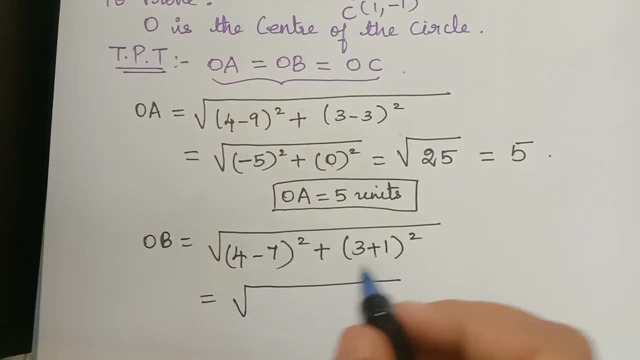 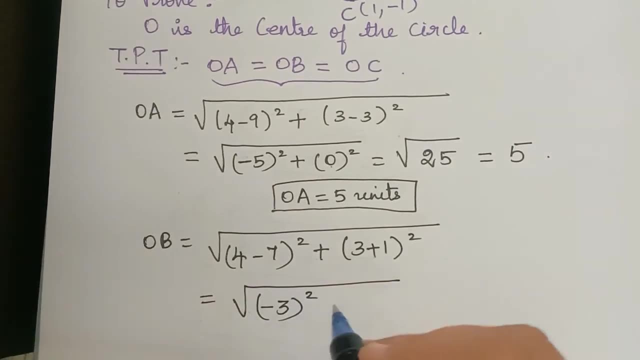 to square root of now. what is 4 minus 7 minus 3, so minus 3. the whole squared, plus 3 plus 1 is 4, so 4 the whole squared. so that is equal to square root of now. minus into minus will become plus 3. 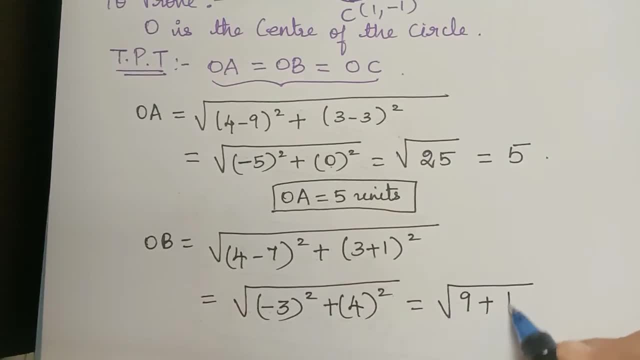 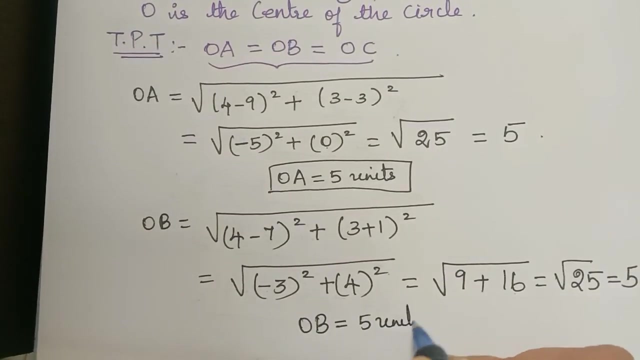 3 times is 9 plus 4, 4 times is 16, and so that is equal to square root of 25, because 9 plus 16 is 25.. And which is equal to 5 again. so therefore ob is equal to 5 units. so we have found ob here. now next: 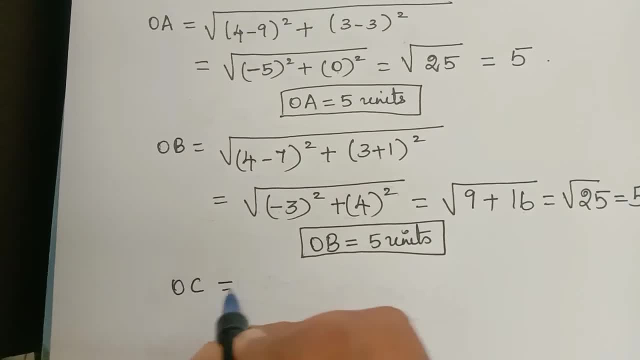 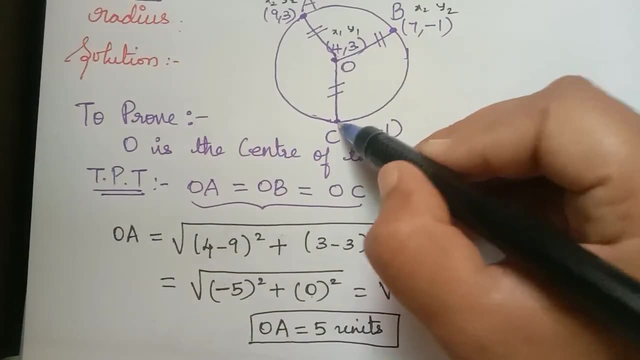 we shall find oc. so oc will also be in the similar manner, square root of now. what is oc now here? this will be x1, y1, now c is this coordinate, so this will become x2, y2 now. so it will be 4 minus 1, the. 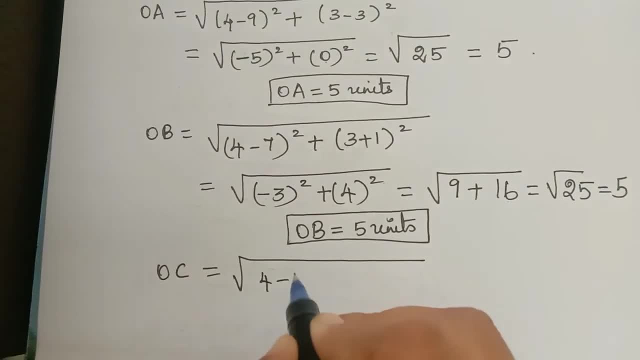 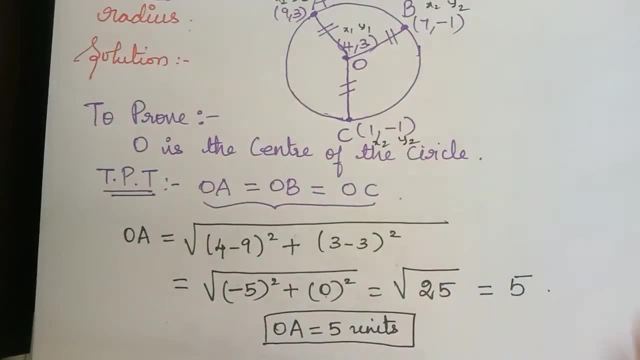 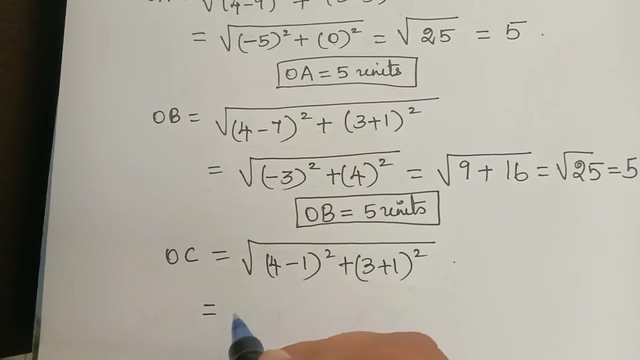 whole squared: 4 minus 1, the whole squared plus. now what about the y coordinate? it is 3 minus of minus 1, so it will become plus 1. so 3 plus 1, the whole squared, and so that will be equal to square root of what. 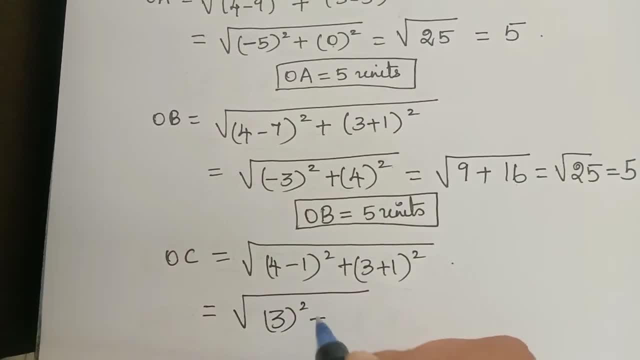 is 4 minus 1, it is 3. so 3 squared plus 3 plus 1 is 4. so 4 squared, which is equal to square root of again 3, 3's are 9, 4, 4 times is 16, and the sum: 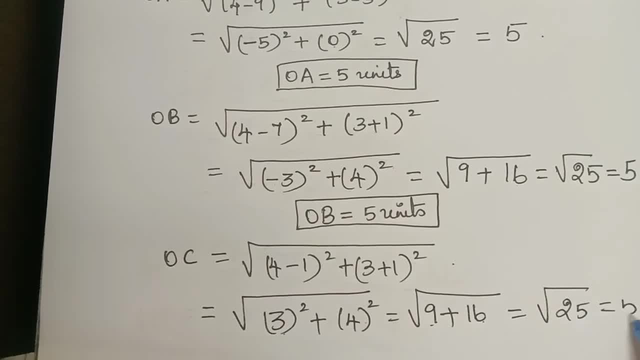 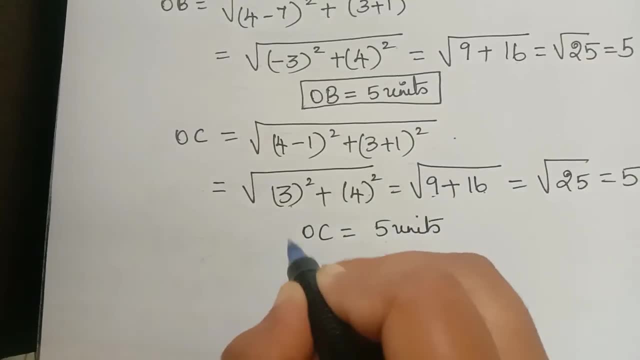 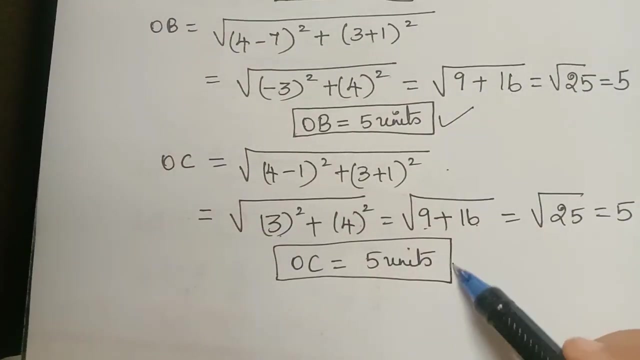 Of these, 2 is 25, and so that is equal to 5 again. so therefore, oc is equal to 5 units. so hence we have proved that o a is equal to ob, which is equal to oc, which is equal to 5 units. so therefore, o a is equal to ob, equal to. 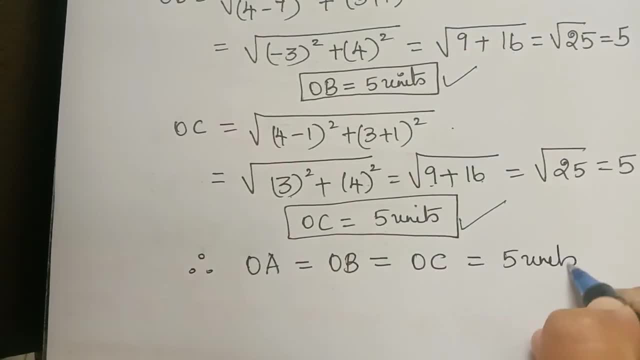 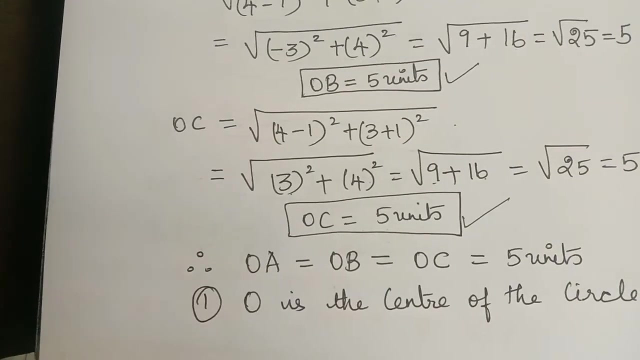 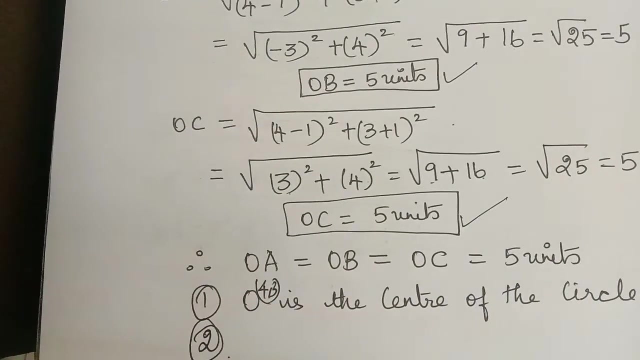 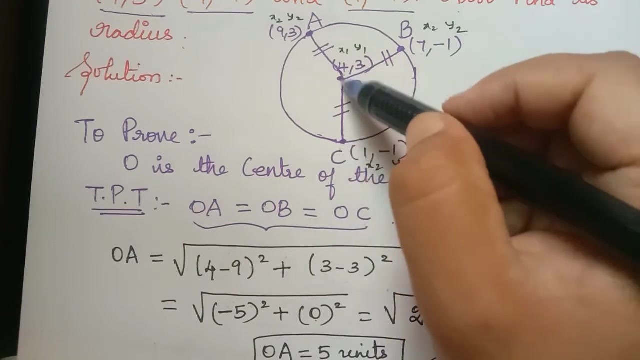 o c, which is equal to 5 units. so first, we have first proved That O is the center of the circle. so o is the center of the circle. what is o point o is 4 comma 3. so 4 comma 3 is the center of the circle. that is what we have proved. second thing: they are asking us to find the radius. but actually what is radius? radius is nothing but o, a or ob or o c. so all these are radius of the circle and we have got that to be equal to 5 units. And so therefore the radius of the given circle- so radius of the given circle is- equals to 5 units. so hope you have understood this problem, thank you. 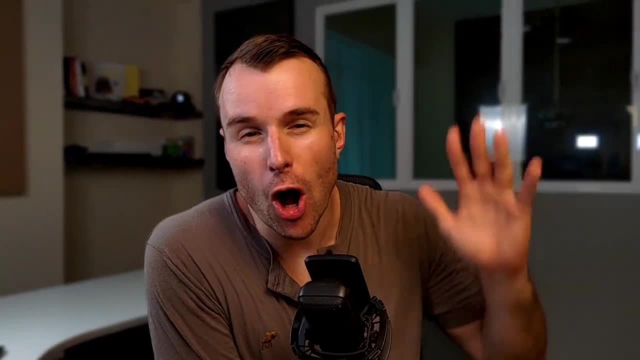 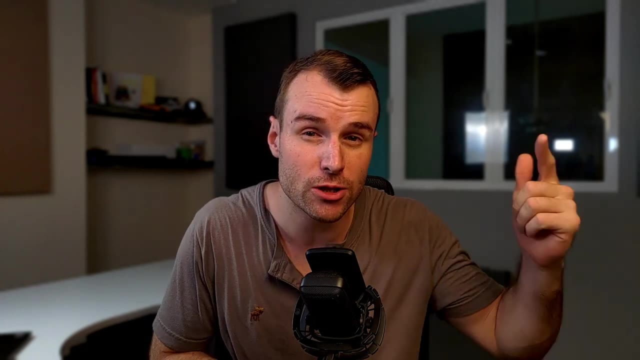 The cat in a dog's world meme coin. the Mew token almost doubled today in a market that's pretty much silent. What's going on here? What's behind this rally? How much longer could this last? Let's have a look at data most people aren't looking at. Let's dive deep into the blockchain.